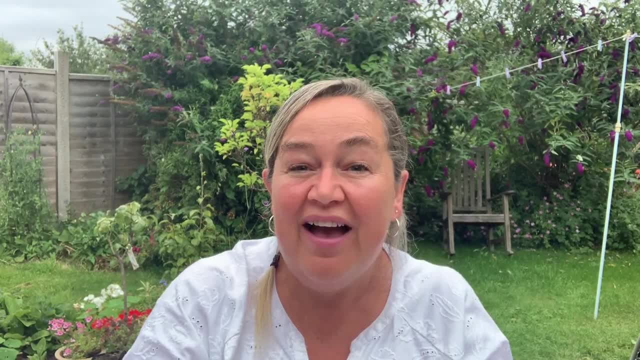 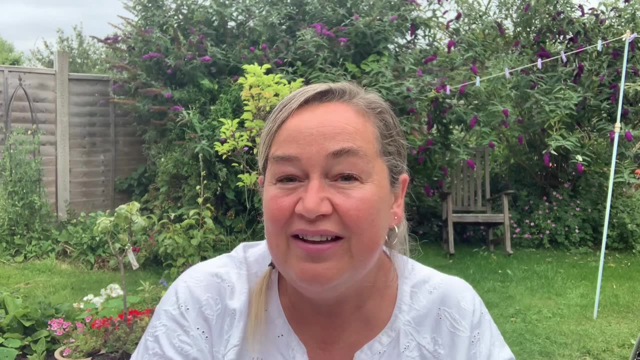 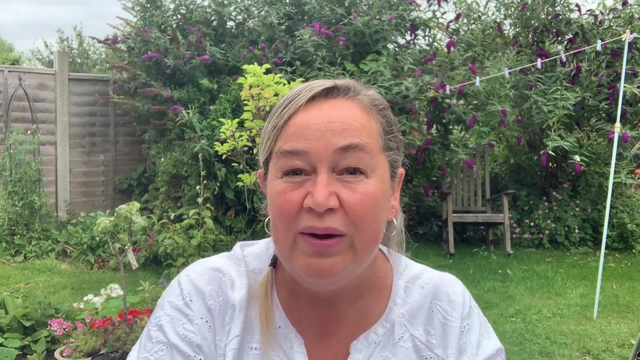 Hi everyone, I'm Becky and today I'm going to show you how to make a nature craft window. Making nature art is one of the most relaxing things you can do. Nature always makes us feel more zen and less rushed, and when we craft or make art, we get into that state of flow where 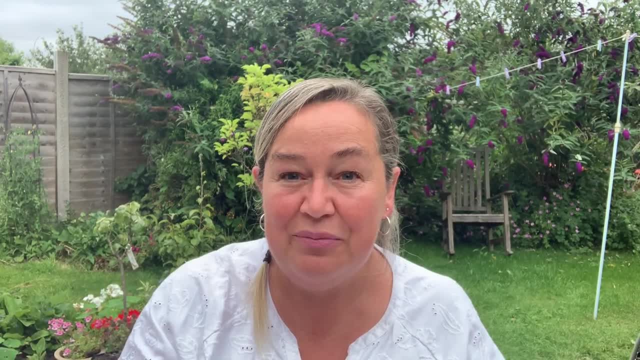 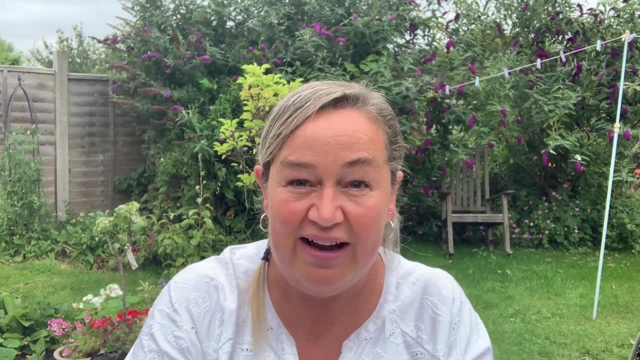 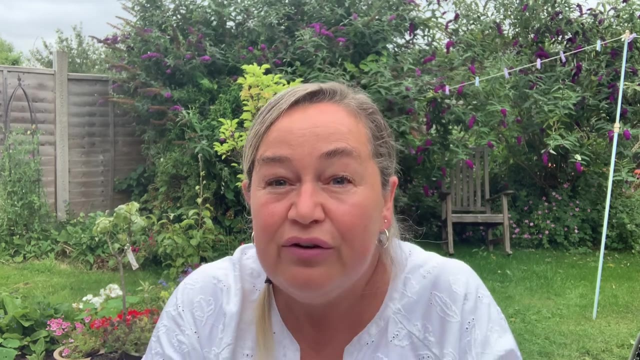 our worries are all forgotten and we're just entirely in the moment. So nature and art combined are just a winning combination. if you want to feel less anxious, Nature windows are gorgeous. Let me tell you how to make them. it's super simple. You need four sticks to make a frame. 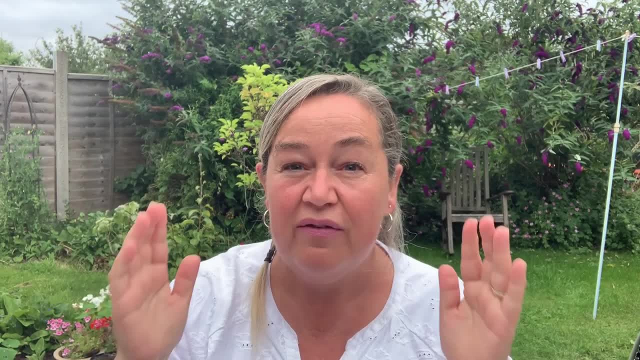 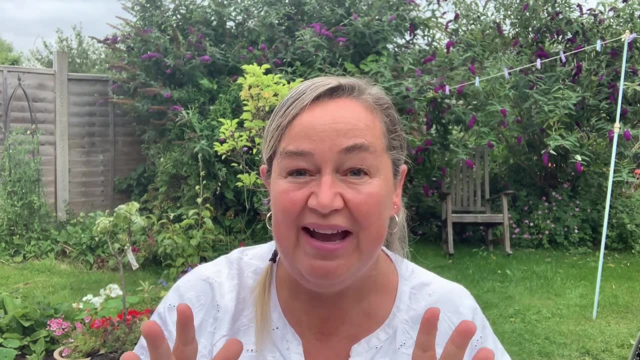 so preferably the same sort of length. you can always break them off and you want them to be straight. So you've got your four sticks, you're going to lay them on the ground and make a window. Okay, when you've got your window, you're going to fill it. so imagine it like a picture frame. 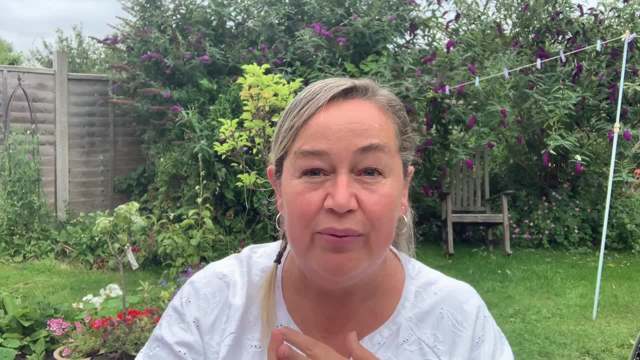 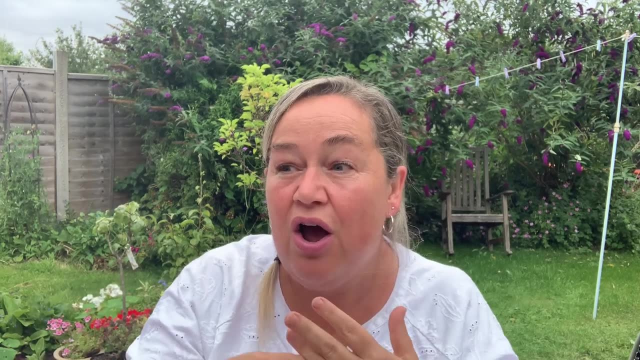 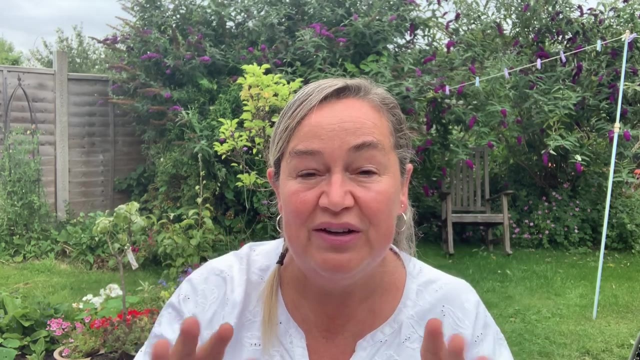 and you can use shade. You can use shells or stones or pebbles. you can use leaves or twigs. you can use flowers that you've found- not, obviously, that you pick, but ones that you've found on the ground- or petals and you. 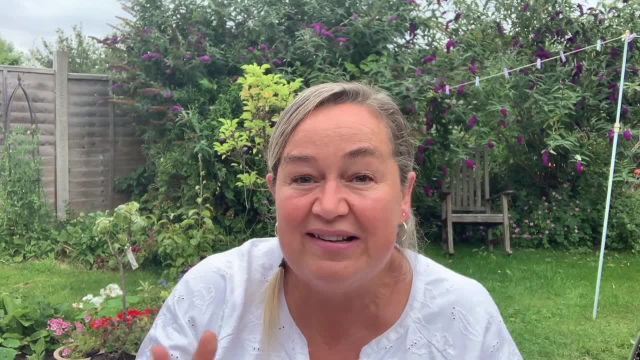 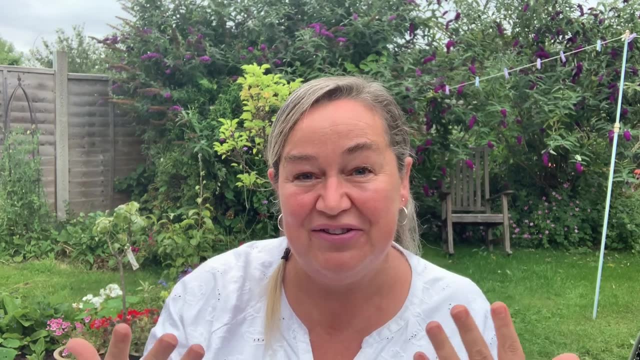 just can make a beautiful picture inside your frame. Now you can do this in the garden to bring yourself pleasure. you can do it on the park, where you leave it, and imagine the strangers that are going to stumble across it and find it and just love it. 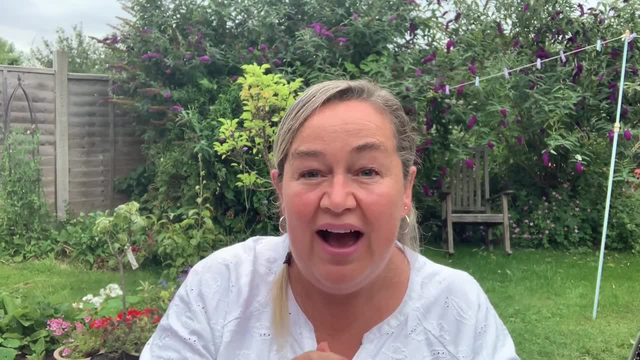 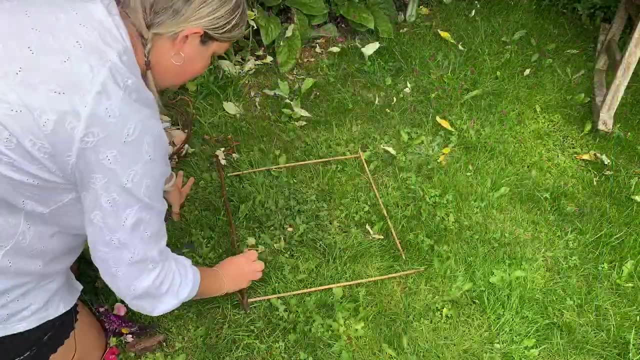 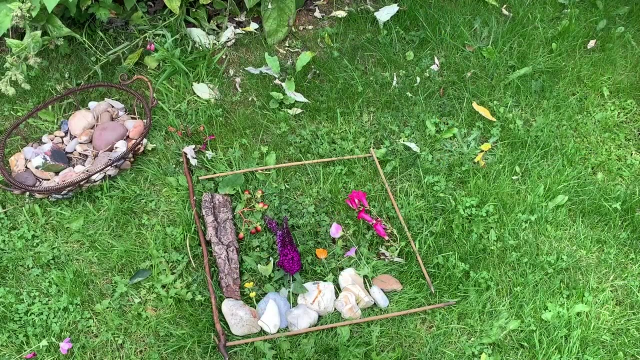 You can leave it on the beach, for example. just a little gift for you out into the world. but I guarantee you'll feel calmer if you make one of these. So let's have a go. Obviously, I'm not that quick when I do it normally, but there you can see. 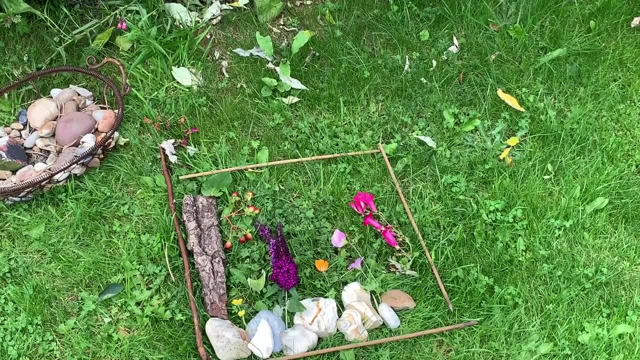 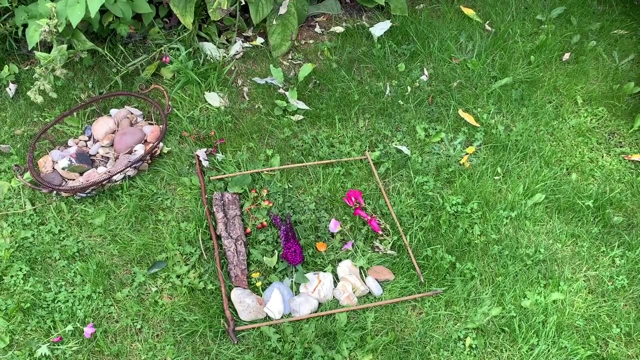 is my little picture. Now you can make a picture of a butterfly, of a landscape, like I've done, or you could just make a mandala shape or just some kind of random pattern. really doesn't matter, But can you imagine someone just walking along and stumbling across a nature window? that? 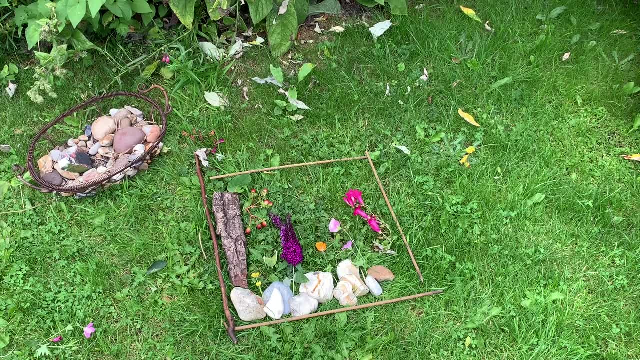 you've left out there for them. Isn't that just a lovely thought. Anyway, I really hope you have a go at making one of these and that it helps you feel as calm as it makes me feel.